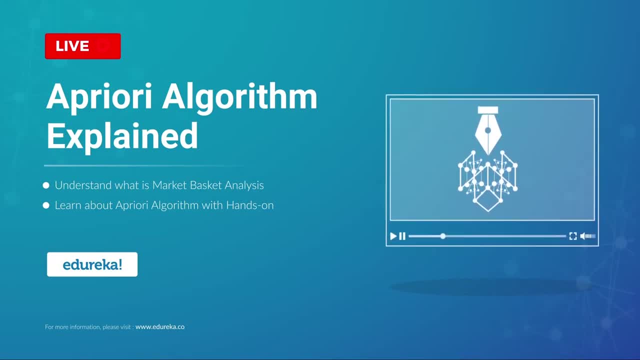 for the confirmation everyone. So my name is Neeraj Kheria and I have been working in this IT industry for more than 13 years now. So the main agenda for today's session: we are going to discuss on the market basket analysis here, how the association rule mining. 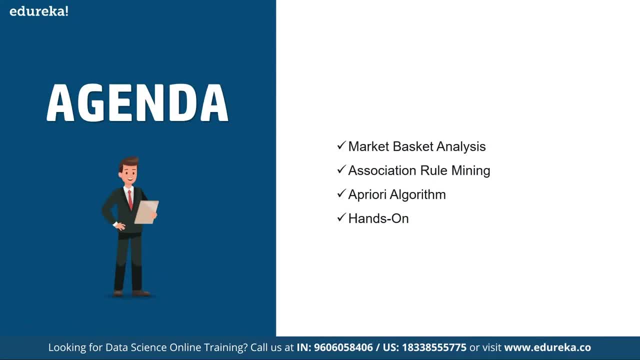 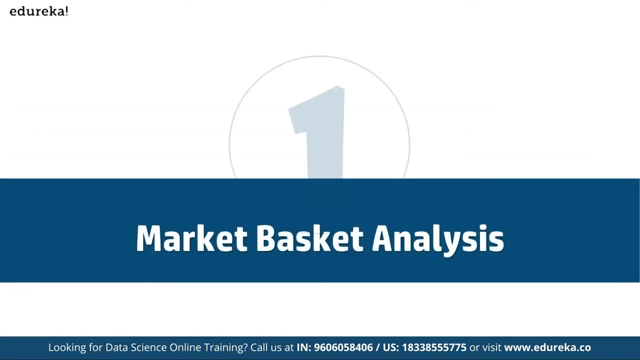 works and how the Apriori algorithm works. A small question that we can start with is: has it ever happened that you are out to buy something and you end up buying a lot more than you have planned? So this normally happens in the marketplaces, correct? So it's a phenomenon. 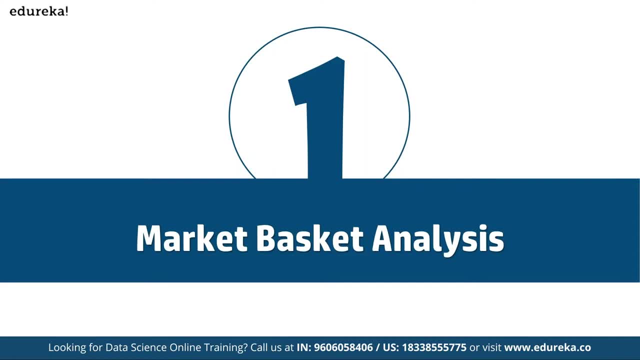 that we are going to discuss on the market basket analysis here, how the association call as the impulsive buying, and big retailers take advantage of machine learning and Apriori algorithm to make sure that we tend to buy more, And that's what we have defined as a. 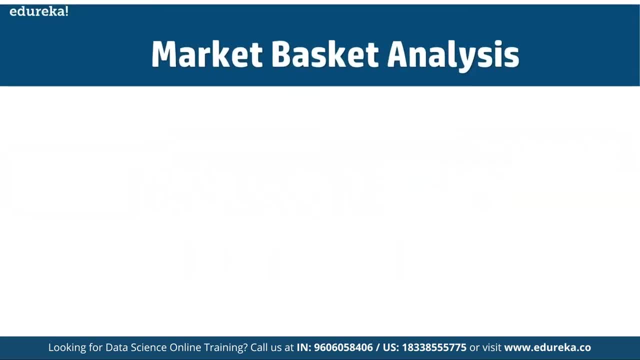 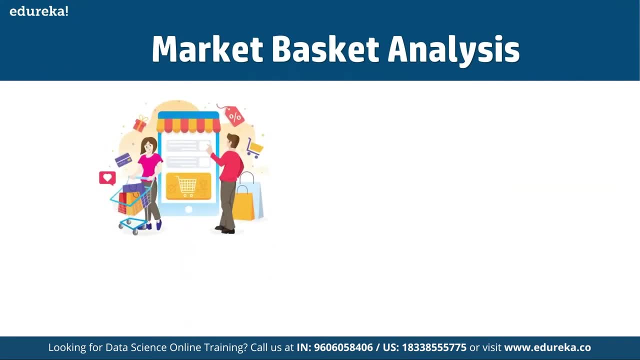 market basket analysis. Now, first of all, let's discuss on that. So in today's world, the goal of any organization is to increase the revenue. And can this be done by pitching just one product at a time to the customer? The answer is clearly a no. Hence the organization began mining data related to frequently bought 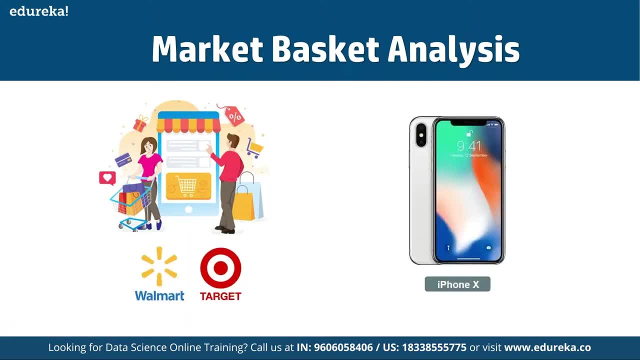 items. So market basket analysis is one of the key techniques used by large retailers to uncover associations between items. So they tend to find out the associations between different items and products that can be sold together, which gives assisting in right product placement. Typically it figures out what products are being bought together and organizations can place. 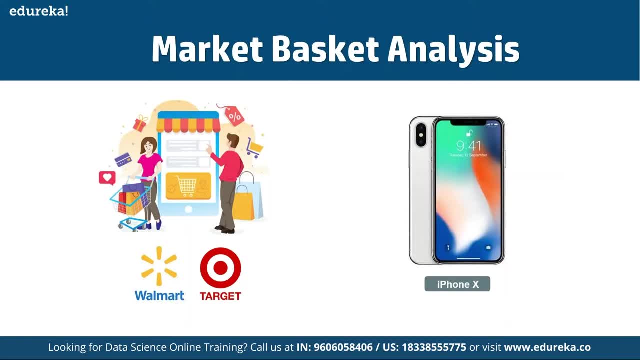 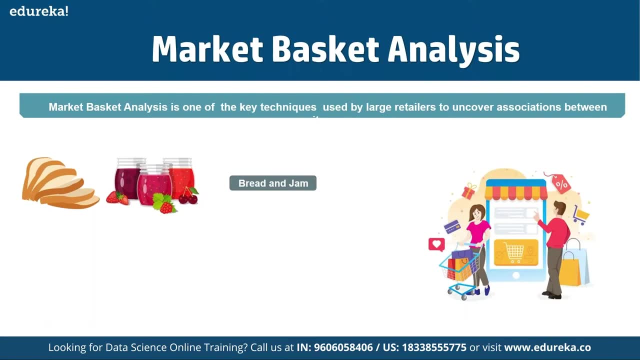 products in a similar manner. Now let's understand this better with an example. Let's say we have people who buy bread usually buy butter too. So the marketing team at retail stores should target customers who buy bread and butter and provide them an offer to them, so that they buy the third. 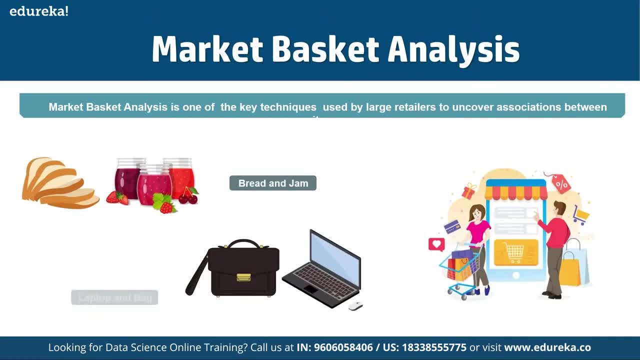 item that we have eggs or any kind of jam As well, Correct. So if a customer buys bread and the butter and see a discount or an offer on eggs, they will be encouraged to spend more and buy the eggs. So this is what market basket analysis is all about. 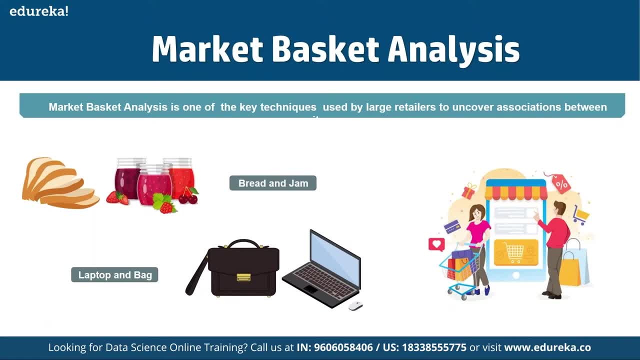 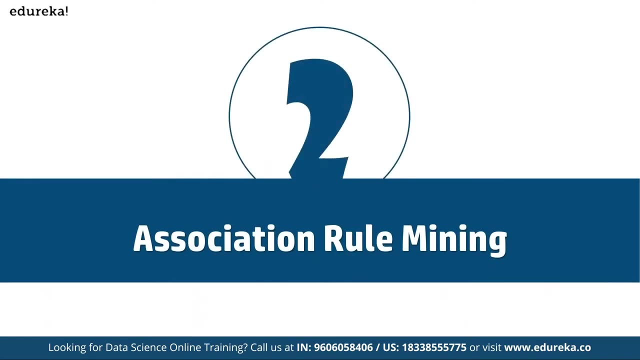 So this is a small example. Let's say, if we take thousand, ten thousand items data of our supermarch to a data scientists, just imagine the number of insights we can get out of it. And that is why association rules mining is also important to understand. so if you talk about association rule mining, then 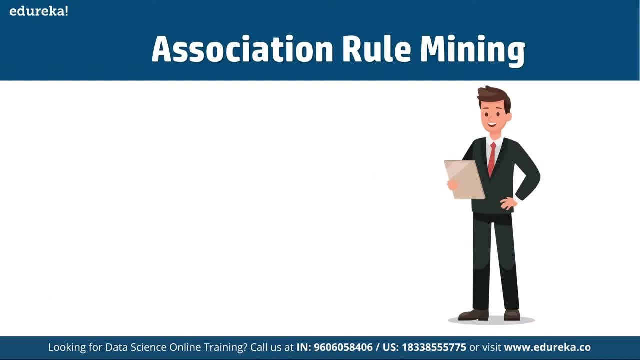 association rules can be thought of as an if then relationship. suppose we have an item a, so item a is bought by the customer, and then the chances of an item b being picked by the customer to under the same transaction id is found out. so here we have simple if and then relationship. 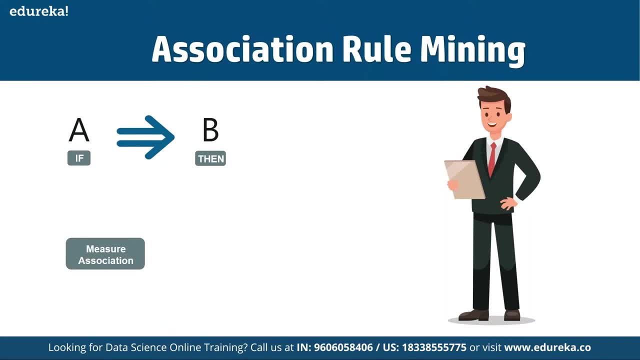 so there are two elements of these different rules. first of all, we have the antecedent as an if so, this is basically an item or a group of items that are typically found in the item sets or data sets, and then we have the consequent. that is then so here we have then. so then is basically: 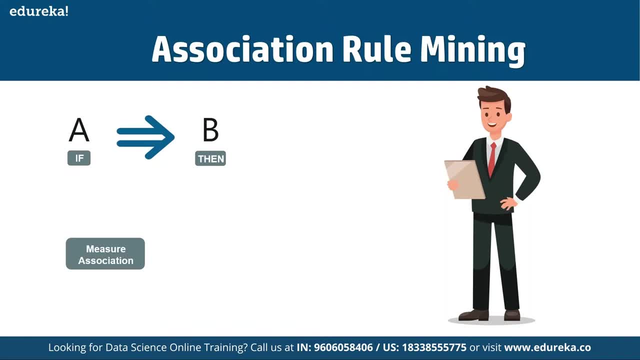 used for. then it comes along as an item with an antecedent or we can say a group of antecedents that we have seen and antecedent we have discussed. it is basically an item or group of items that we found in item sets of data sets. now, 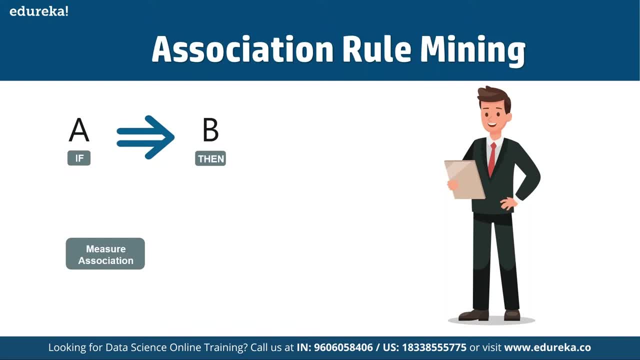 here comes a constraint. suppose we made a rule about an item use. we still have around 9999 items to consider for rule making. as we discussed we have, we are going to make use of 10 000 items. so this is where a priori algorithm comes into play. 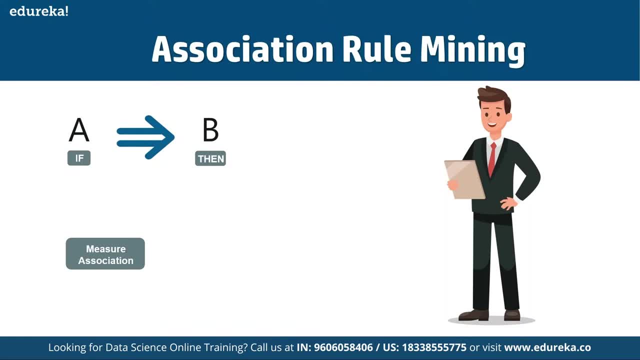 so there, before we understand the apriori algorithm, let's understand the mean mathematics involved in here. so there are three ways to measure the association: we have support, confidence and then we have lift. so as you can measure the association here, we have support, confidence and lift. so support gives the fraction of transactions which contain. 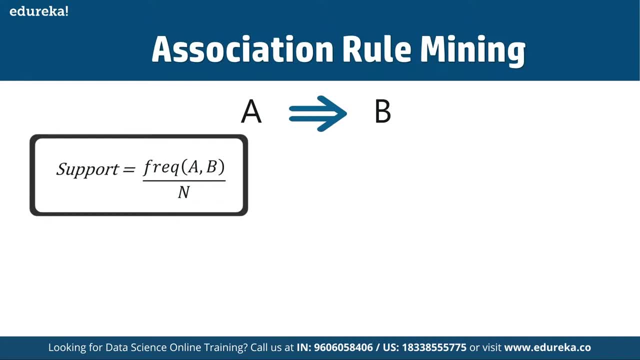 item a. suppose. if we talk about support here it is basically a frequent, the fraction of transaction which contains item a and b. so basically support tells us about the frequency for the against that we can say frequently bought items or the combination of items bought frequently by using. 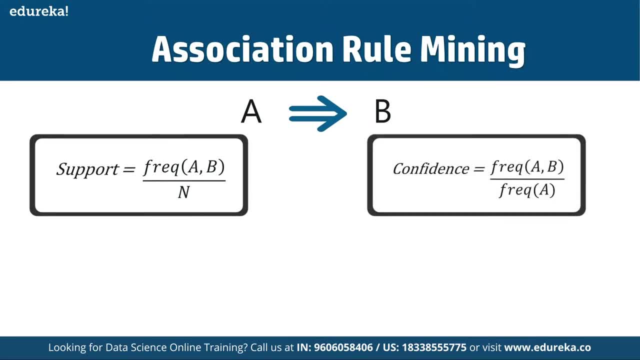 the support. so with this we can filter out the items that have a low frequency. then we have confidence. so it tells us how often the items a and b occur together, given the number of times a occurs. so typically, let's say, when we work with the apriori algorithm, we define different terms. 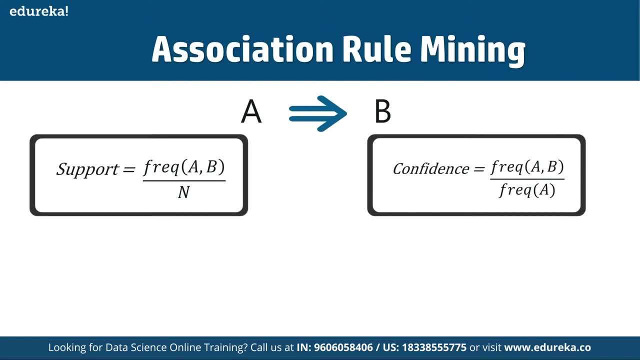 accordingly, but how exactly we have to decide the value. that's the main question. and, to be honest, there is not a specific way to define these terms. suppose we have assigned the support value as 2.. now what is? what exactly this means is until and unless the item frequency is not. 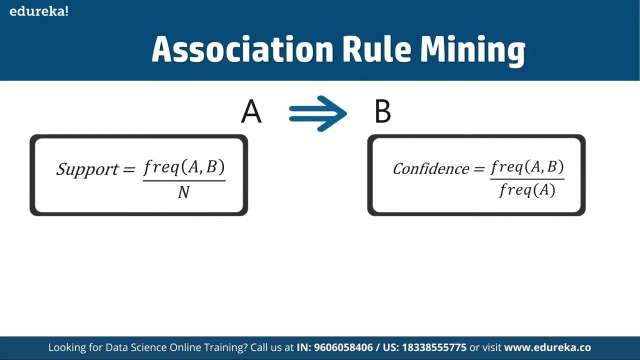 two. so here we define support as two. so until unless the item's frequency is not two percent, we will not consider that item for the a priori algorithm. so this makes sense, as considering items that are bought less frequently is a waste of time because, let's say, if only two percent of users are 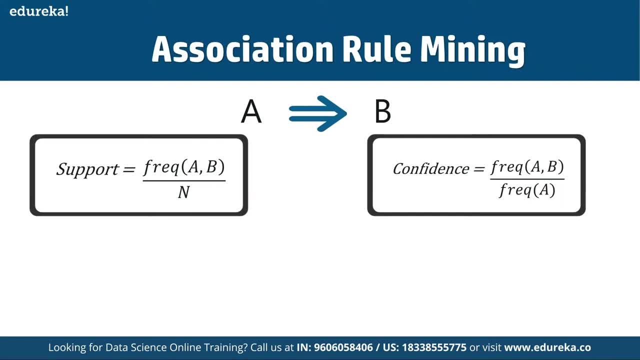 you are buying this item along with the item that they have bought, then obviously they cannot use it. we cannot even consider is for the a priori algorithm that we are going to work on here now. suppose after filtering, we still have around five thousand items left now creating. 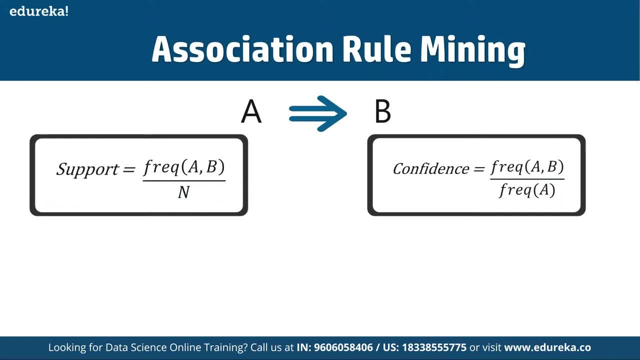 association rules for them is a practically impossible task for anyone, and this is where the concept of lift comes into play. so basically, lift indicates the strength of a rule over the random occurrence of a and b, and it basically tells us the strength of any given rule here. 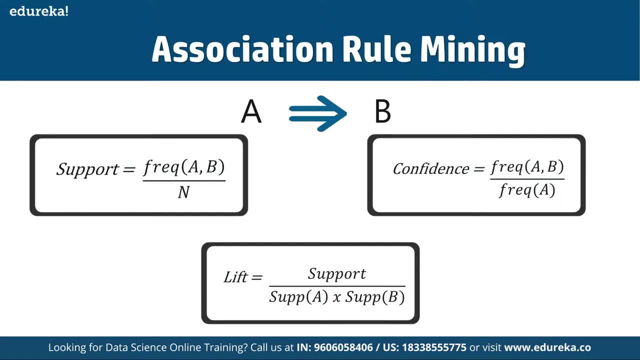 so if i'm finding that out, we have simply divide support with the by the, the support by the support of a and then support of b. so focus on the denominator. it is the probability of the individual support values of a and b and not together. so lift explains the. 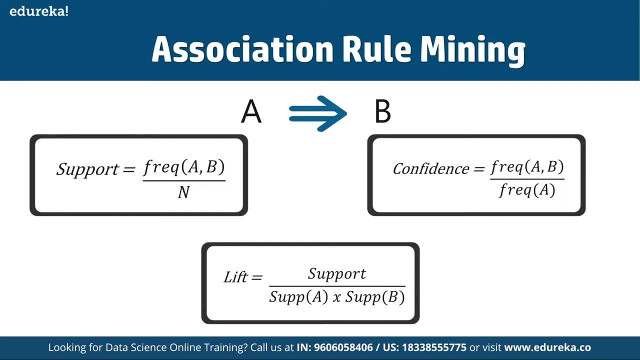 strength of a rule. so more the lift, more is the strength. let's say a as opposed to. we can say for a is to be so if a, if then relationship. so if you talk about if then relationship for a, b, then the lift value is four. so first let's say for this relation the lift value is four, here that 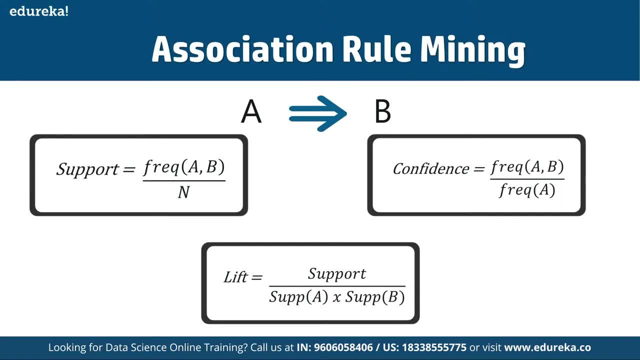 means if you buy a, then the chance of buying b is four times if the lead value is four, or we can say it's four times if the value here is two, then it is two times, and so on. as a part of the lift. values are fine, so let's get started with the a priori algorithm. 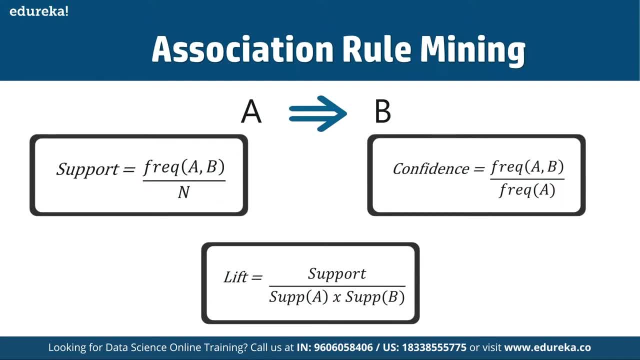 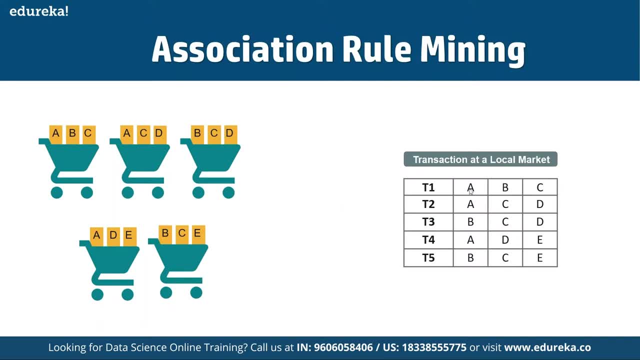 now let's see how exactly it works. all right, so now let's discuss on the concern. this is what we discussed here: the transitions at our local market, and here we have abc for in transition two, we have acd in transition. three, we have bcd in transition four, we have ade and then we have in transition. 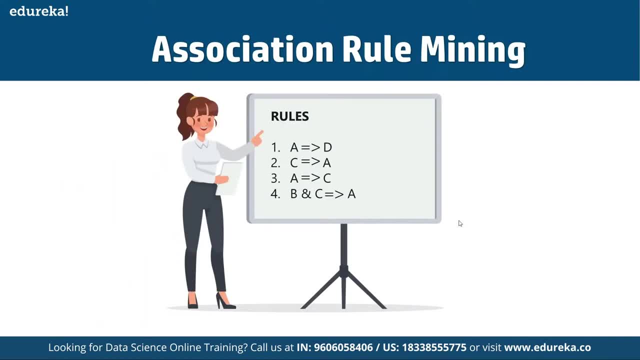 five. we have bcd. so let's say here: if you find out the entire rules here, then a. if a, then again they are going to purchase d. if they buy a seed, again they have the option of going for a. if they buy a, then they have the option of going for c, and if they buy b and c together then they are going. 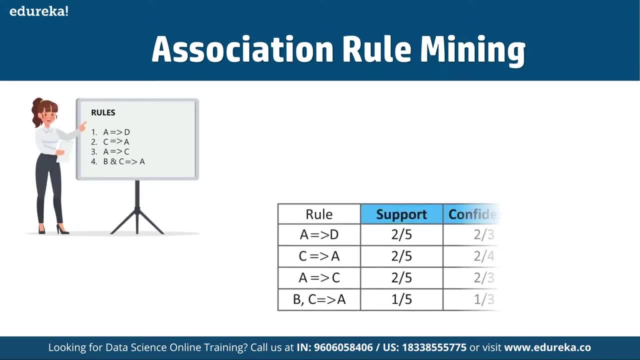 to buy by a as well, and then, same way we can find out the support. so again, for if a is for those who are purchasing a, the probability of buying d, it is some. in terms of support it is two by five, in terms of confidence it is two by three and in terms of lift it is ten upon nine, whereas for c. 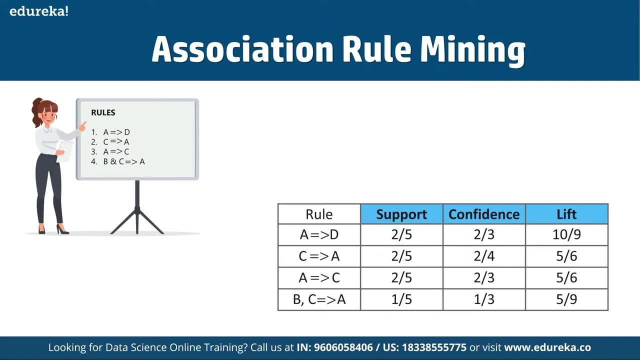 for a. that means what is? what is the possibility that those who have purchased c will be buying a. so you can find the support as two by five, confidence at two by four and lifters, five by six, same way for c and same way for bc and a. so we can see how the probability is going to be. 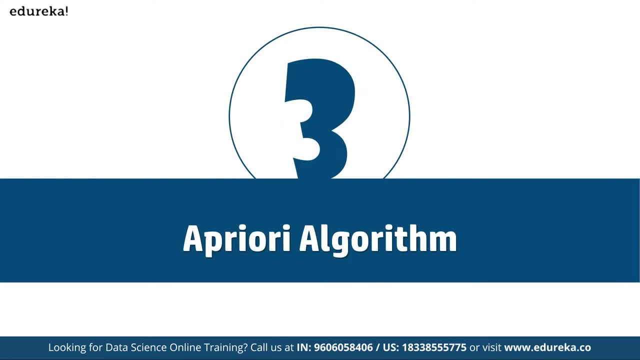 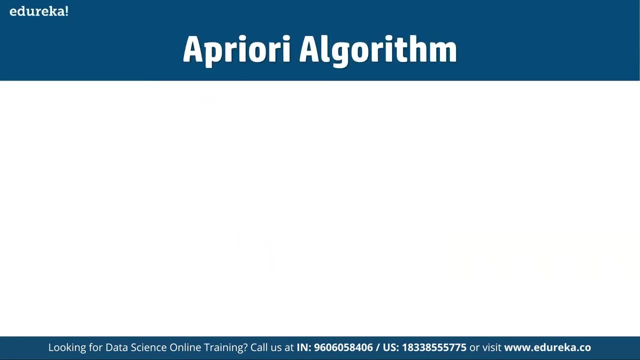 distributed as we, as we find out the possibility of one product to be bought over the other. all right, so now let's assume further on the apriori algorithm part. so aprio re algorithm uses frequent item data sets against item sets or data sets to generate the 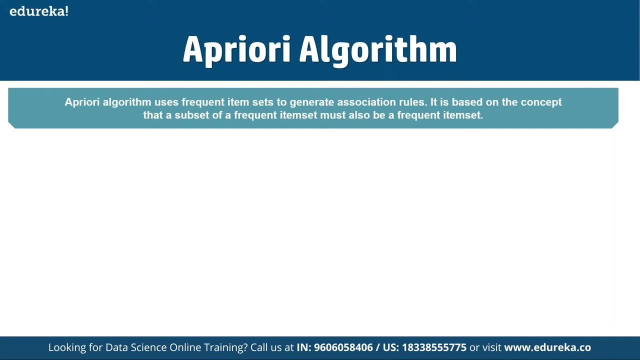 association rules. so it is based on the concept that a subset of a frequent item set must also be frequent item set must be a frequent item set, and frequent item set is an item set whose support value is greater than a threshold value that we have support. so let's say we have. now we're 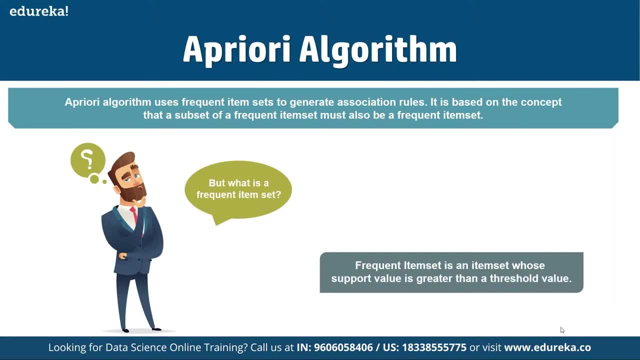 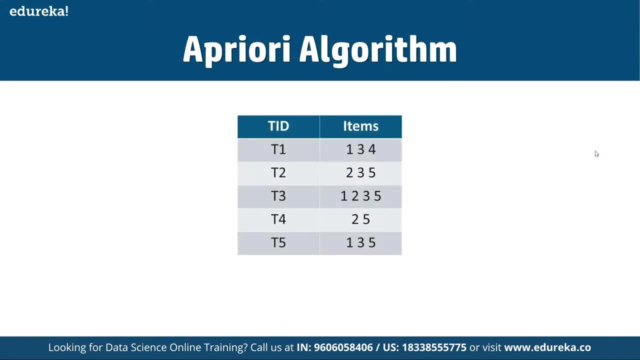 what exactly a frequent item set is what we discussed just now. it's an item set whose support value is greater than a threshold value. all right, so now, if we talk about a simple example, now here we can, let's say, we have the following data of a store here, so we have the transition. 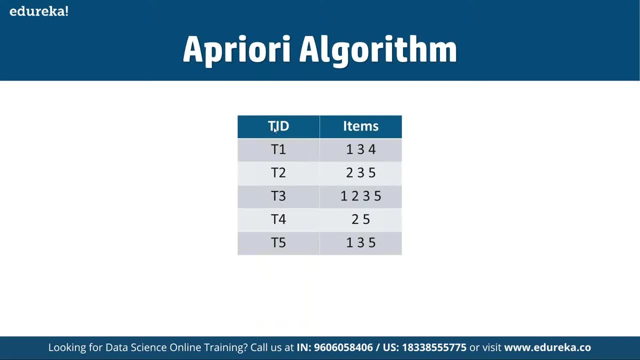 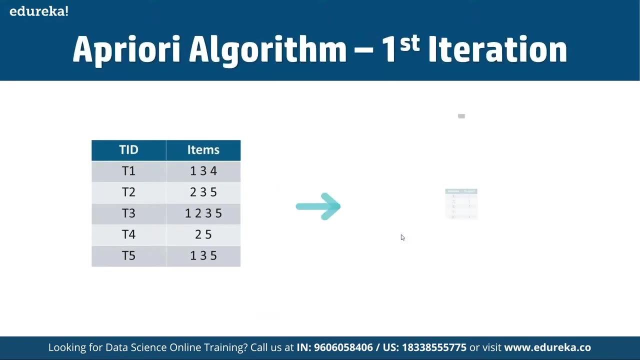 id here and then we have nine items. so so here we have these. one are transaction ids and here we have the items. so in transaction one we have one three four, two three five, one two, three, five, two five and one three five. so if we talk about the first iteration now, let's assume the support value is two, and then we can. 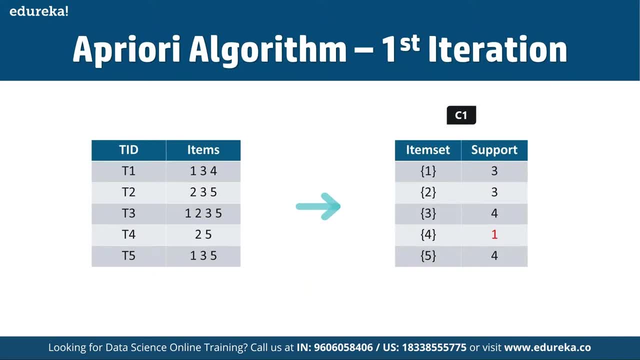 create the item sets of the size one and calculate their support values, as you can see here. so, as you can see here, the item four has a support value of one, support value of one here, which is less than the minimum support value. so we are going to discard four in the upcoming iterations and we have 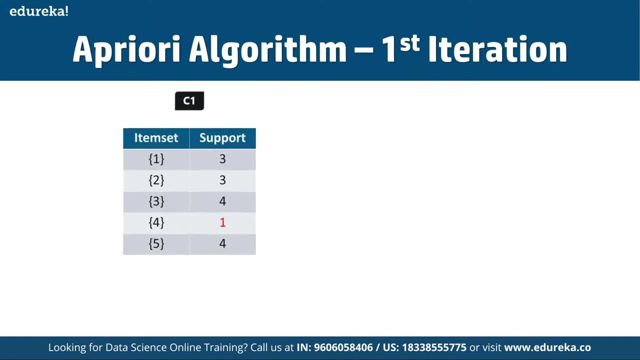 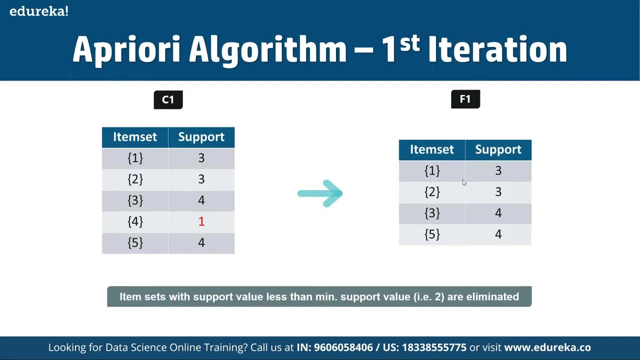 and that's how we can have the final table defined here as the fn. so here we are going to discard the value as four and then we are going to have the final value to be given, given to us. so the item sets your support value less than minimum support value, that is, two are going to be eliminated. 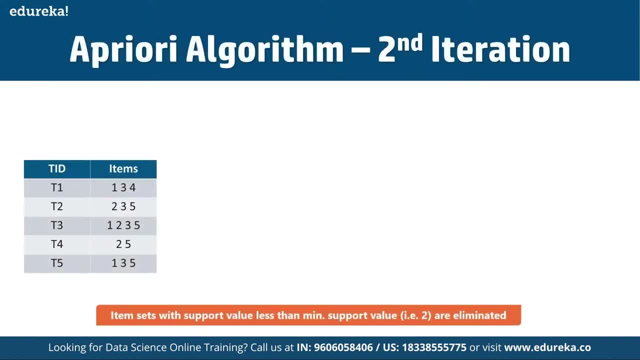 next we are going to create the item sets of size 2 and calculate their support values. so all the combination of item sets in f1 are used in the iteration here. so here we have c2 and then we have the f1 here. so basically, here we are going. 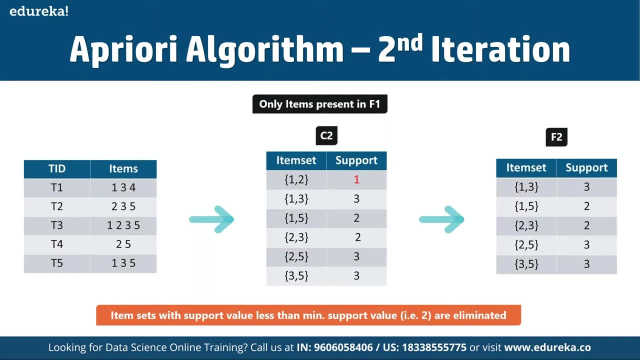 to make use of the entire iteration here, and item sets having support less than two are eliminated again, and in this case we have one and two right. so let's now understand what exactly we mean by running and how it makes apriori one of the best algorithms for finding the frequent item sets. 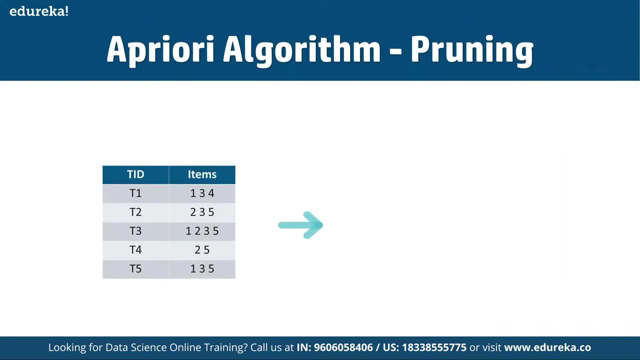 so if we talk about pruning, then we are going to divide the item sets in c3 into subsets and eliminate the subsets that are having a support value less than two from this given item sets here. so here we are going to work on the third iteration, so we will discard one, two and three. 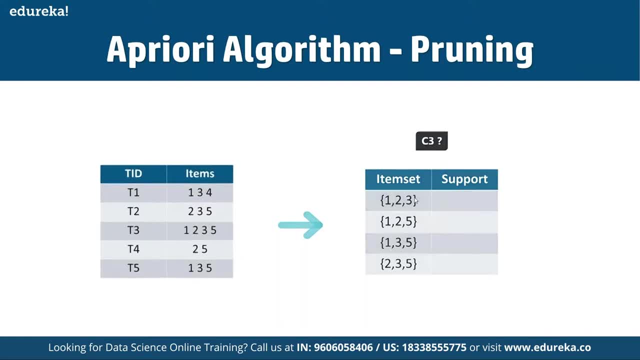 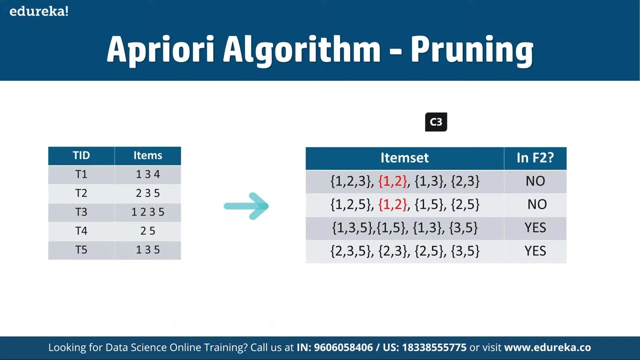 we are going to discard one, two and three, and one, two and five as well, so they both, as they both contain one or two, and this means that again, and this is the main highlight of the apriori algorithm here- so you can see, here we are going to discard one and two and this is the main highlight of this entire algorithm here. 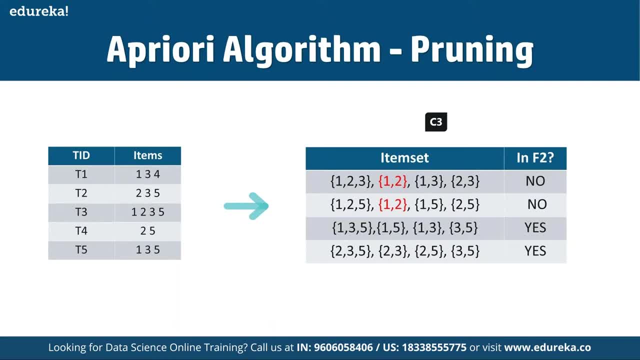 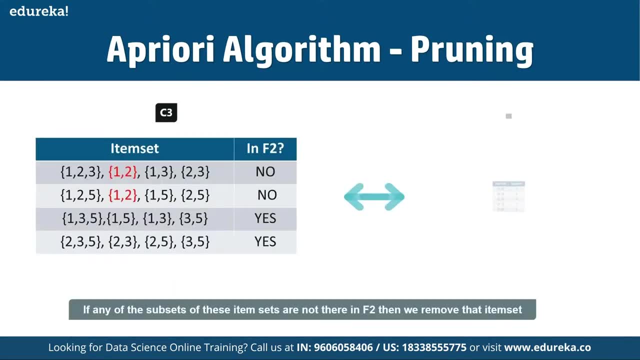 because, again, the one and two is a common thing available in the in these, both data sets right. so this is the main highlight of apriori algorithm here and then, if you talk about the fourth iteration. so now, as you can see, if any of the subsets 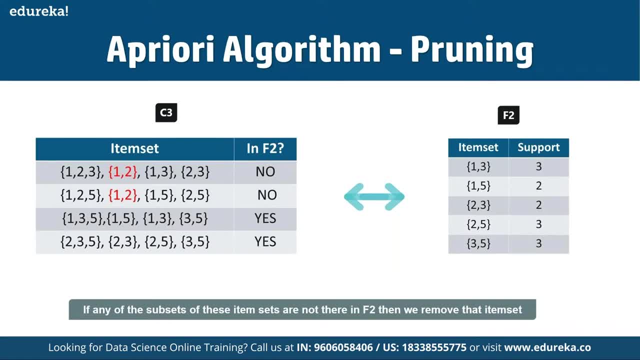 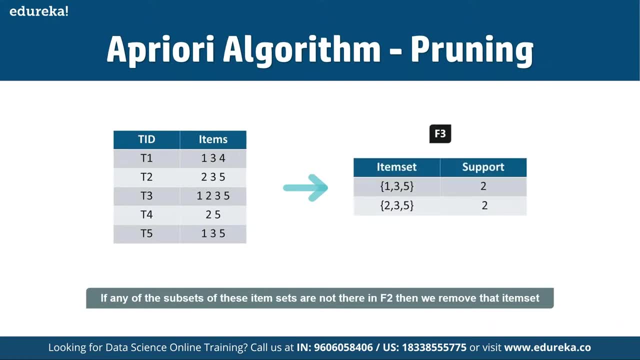 of these items are that are not in f2, then we are going to remove that particular item sets. and then, in terms of the fourth iteration, let's suppose here we have the transition id and here we have the item set and support available. so, since the support of this item set is going to be less than two, 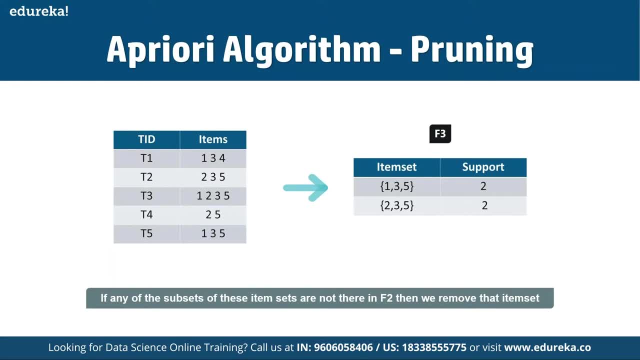 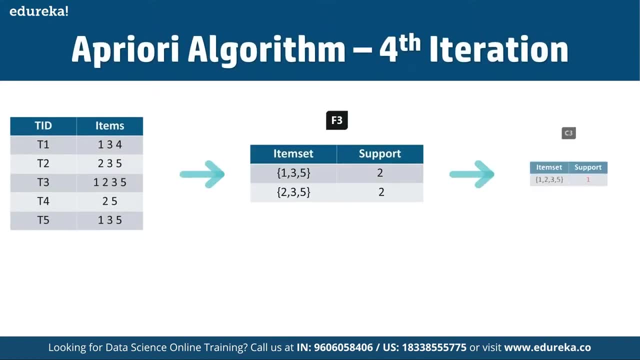 so we will stop here and the final item sets will have is the f3 one. and now, still now, we have not calculated the confidence value yet. so again, this is something that we have to keep in mind. so with the following item sets, that means for one we have one, three and five, and subsets are one, three, one. 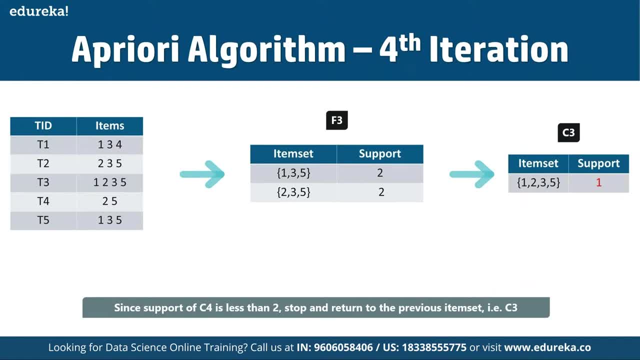 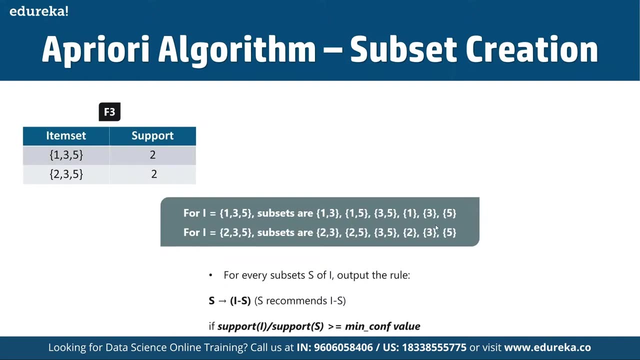 five, three, five, one, three and five, whereas for item sets, one again we have two, three, two, five, three, five, two, three and five itself for the other diamond sets available. so for one we have one, three, five. these are subsets of one, three, one, five, three, five, one, three and five, whereas two, three, five are. 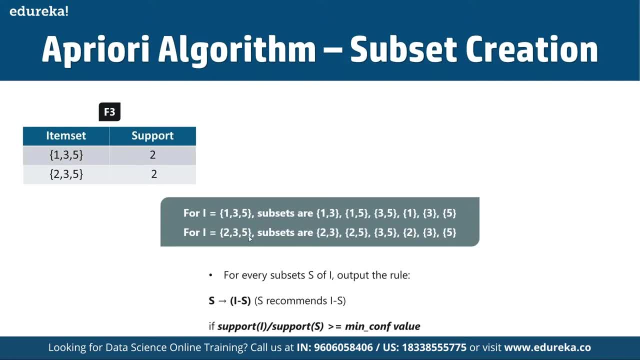 subsets of two, three, three, five, two, five, two, three and five right, and for every subset of i. we have to define the output rule now, when we are going for applying rules here, so we will create the rules and apply them on item set f3. so now, let's assume a minimum. 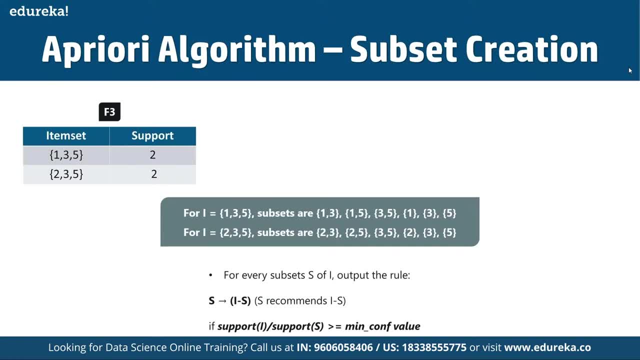 confidence value is 60 percent. so for every subset of whether that we have s of i. so the output rule is going to be: s is going to be recommended, so s is going to simply recommend is, and then we hit support. it is also going to be recommended, so s is going to simply recommend is, and then we hit support. 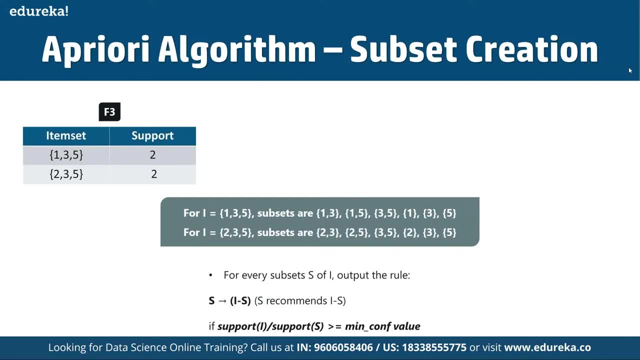 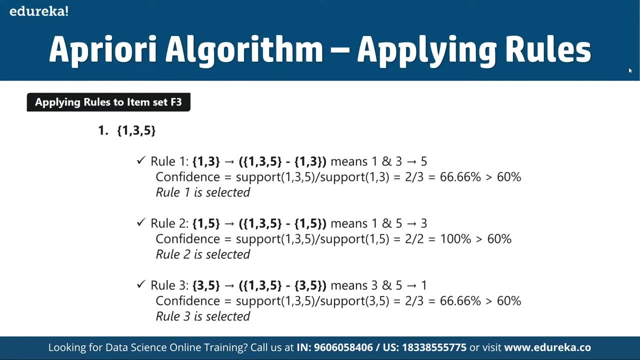 i, and then we can simply divide this by the support cell and to find the minimum confidence value is going to be one to five. so here rule one: here is one. three is again assumption. that means one and three will result to five. that means if a user is purchasing one and three, both the items. 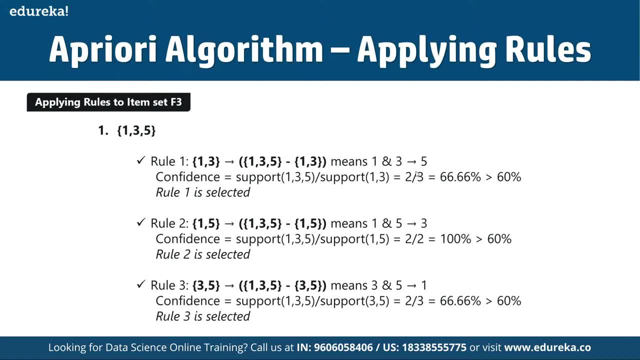 then we have a good possibility of the customer going for the fifth item as well. so here the confidence is going to be support one, three, five divided by a support one three, that is two by two, that is 66.6 percent, that is 60 percent. so here rule one is going to be selected, and in rule 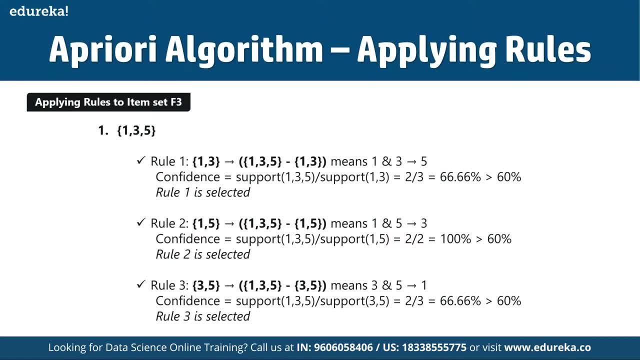 two. we have one five, one three, five minus one five. that means if the people, if someone is purchasing one and five, then they are going to have a good possibility of going for three as well, where we are going to see the confidence and for finding the confidence, we are simply going to again. 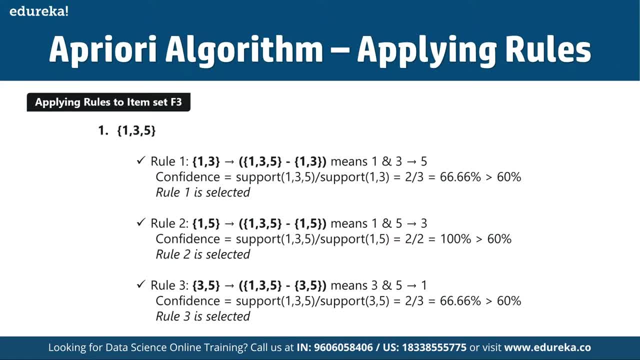 subtract support for one, three, five by support of one, five, that's two by two, and this is going to simply be translated at 100, and which is much greater than 60 as well. and same way in rule three we have three, five, one, three, five, three point five. that means here, if someone is going for purchasing three and five, then they. 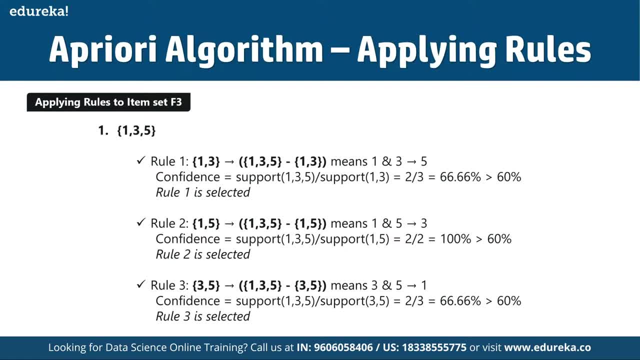 are, then they are holding a high possibility of going for one as well. so here the confidence is support one three five divided by support three five, that we get as 66.6 percent. and here the rule three is going to be selected here, as you can see here. 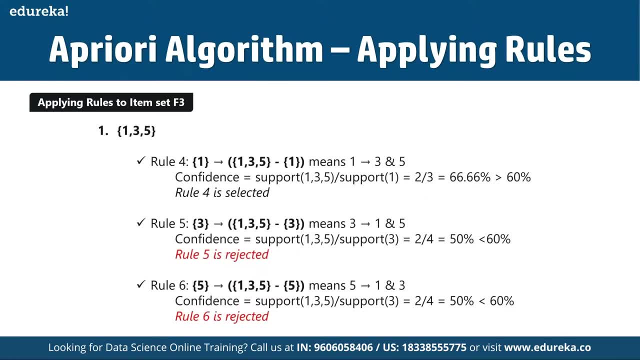 now, upright. now, if you, if you talk about the application of rules here now, when we are talking about this rule here, we can see, whenever the confidence is going to be more than more than 60 percent, defined here, then this rule is going to be selected, as you can see here in this rule five: where what? where those who are 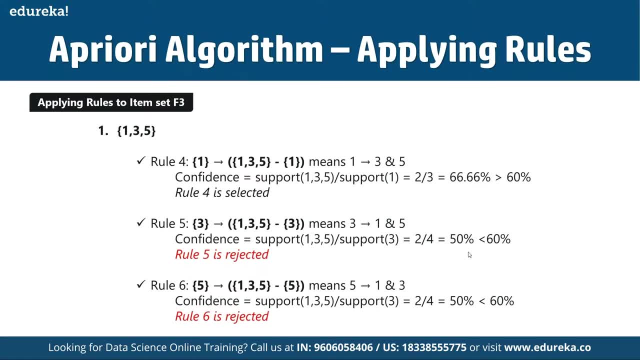 purchasing three, they have a possibility of going for one in five, both. so here the confidence is less than 60 percent, which is why this is going to be rejected. same way for rule six as well. same way here for rule six as well, because here the confidence is going to be less than 60 percent. 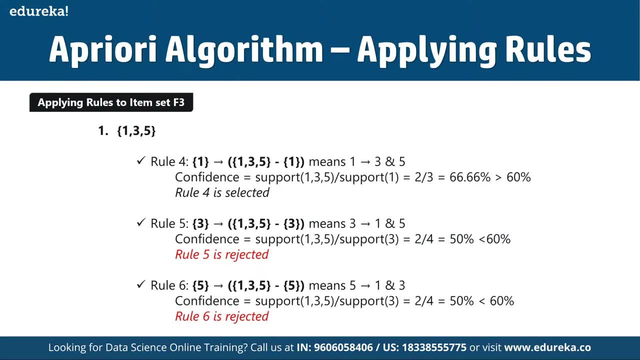 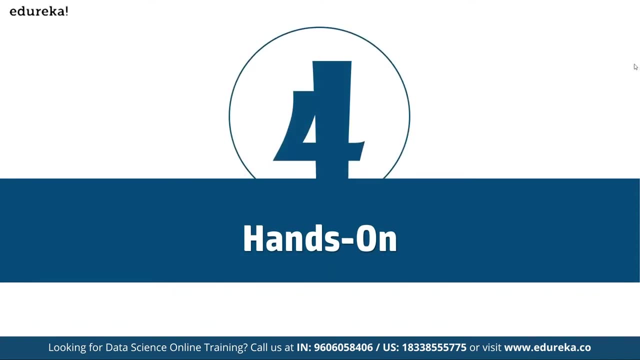 then that's why this is going to be rejected here, correct? because, again here, we have assumed a minimum confidence level for 60 percent, and wherever we are going to get the confidence less than 60 percent, we're simply going to reject that particular model here. all right. so, first of all, 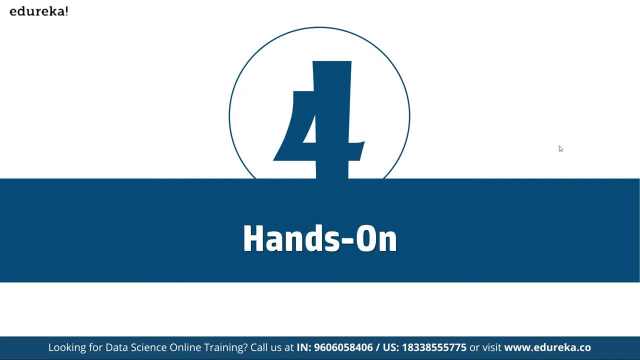 see how we can create rules in apriori algorithms here and the same steps can be implemented for this item. set 2, 3, 5, and then we are going to try it and see which rules are accepted and which rules are going to be rejected and how we can implement the apriori algorithm in python. all right, 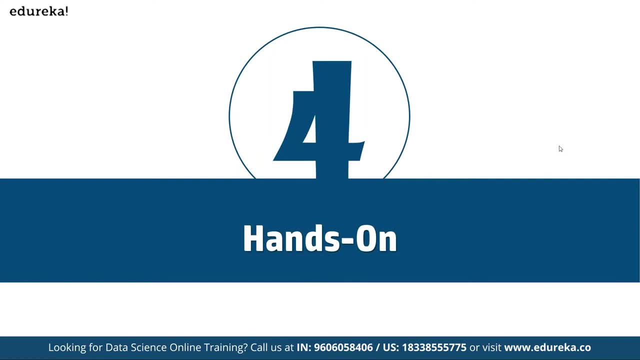 so let's fetch some sample data sets here that we are going to work on. so to get started working on the actual analysis here, we are going to make use of the python id, so we can use any of the id, or we can also make use of the python hormone, ideally to get started. so we are going to make use. 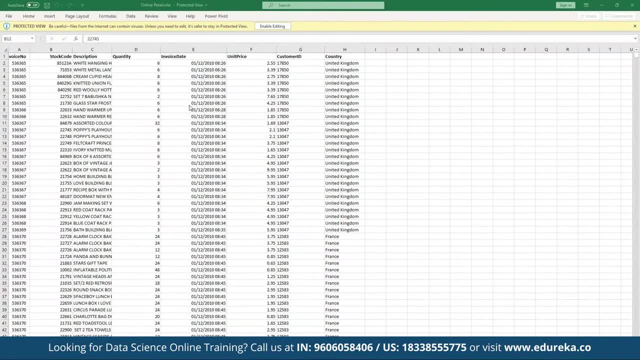 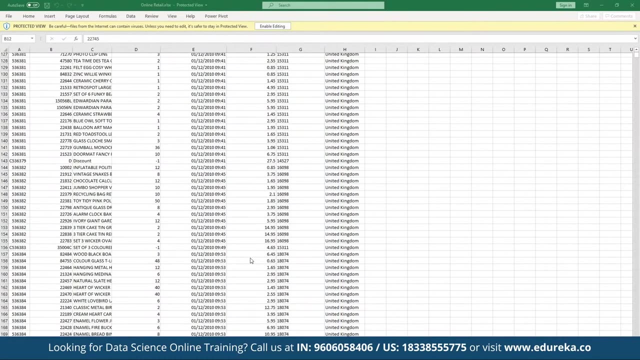 of python. in this file we'll be having the access to the invoice number, we have the stock code, we have description, quantity, invoice date, unit price, customer id and then we have the country. so this is the data point that this is a file that we are going to work on. 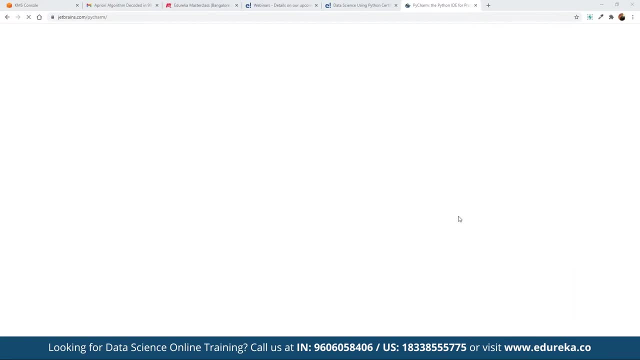 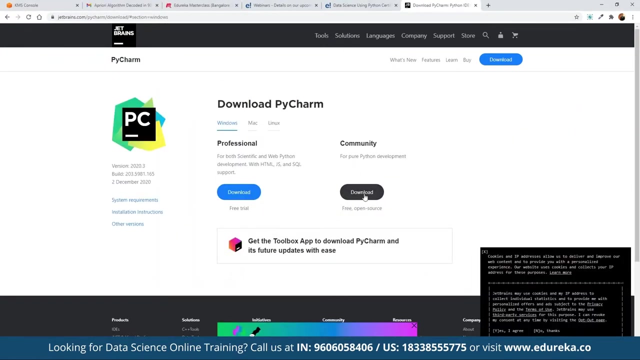 all right. so in the meantime we are also going to install pycharm as our main id. so in case you want to work on python, then we can make use of pycharm id, which is one of the most popular ids for getting started. and pycharm is also offered as a free tool. that means here we get. 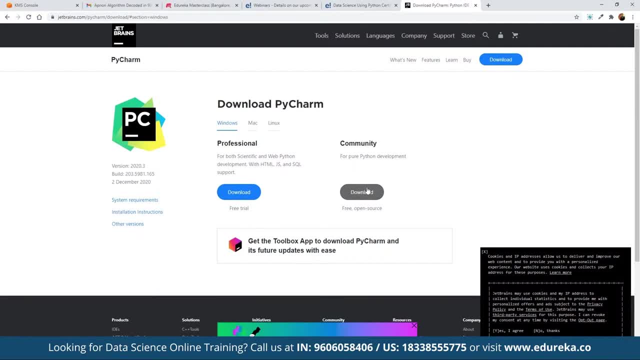 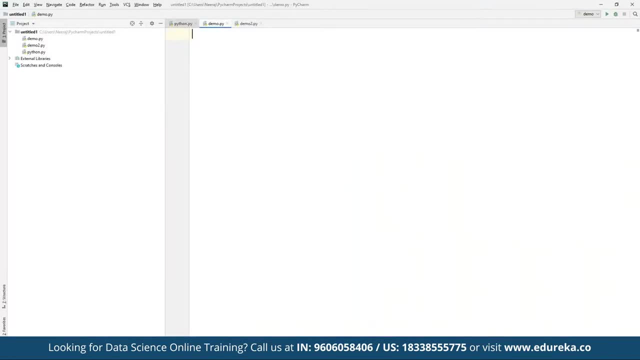 is also offered as a community tool here, so you can use it as a community tool in order to get started. so once we have the access to it, we can open this up. all right, so here we can get started first. first of all, we are going to work on the pandas library, so here we are going. 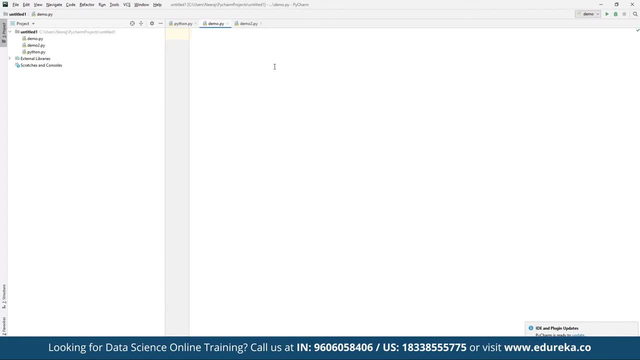 to import pandas and mlxten libraries imported and to import and read the data set. so here we going to choose import and then here we are going to find import pandas and from pandas as pd. so here we go to import pandas as pd and then we are going to use from ml extend. we are going fraud frequent. 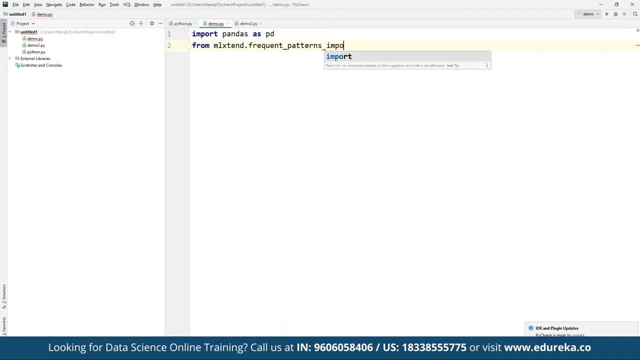 dot frequent patterns. we are going to import a priori and then we are going to use the same from mlx10 dot frequent underscore patterns. we are again going to import association rules. they're going to put up import association rules and then we are going to create a data frame where 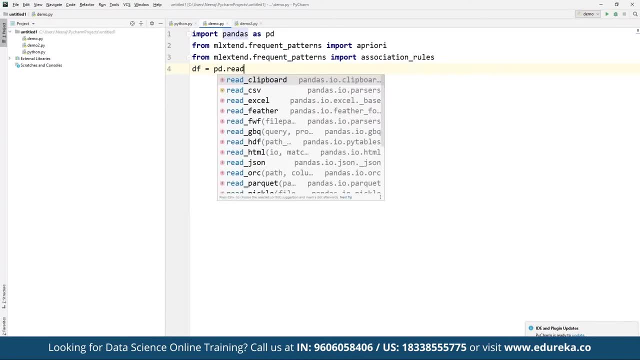 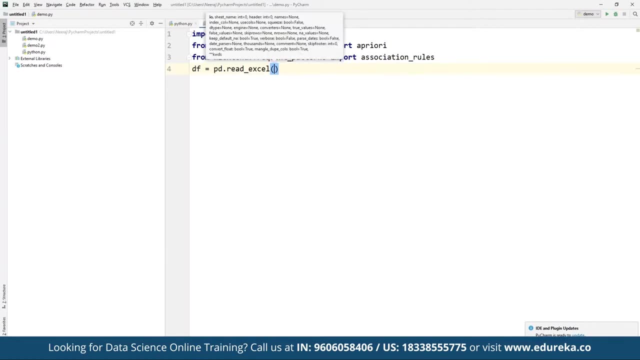 we are going to make use of funda's diary as pd dot read and here we are going to read excel file. if it if it is a csv file, let me define it as read csv and here we can define the path. suppose here the file is currently available in our users location and the users we have it in downloads. 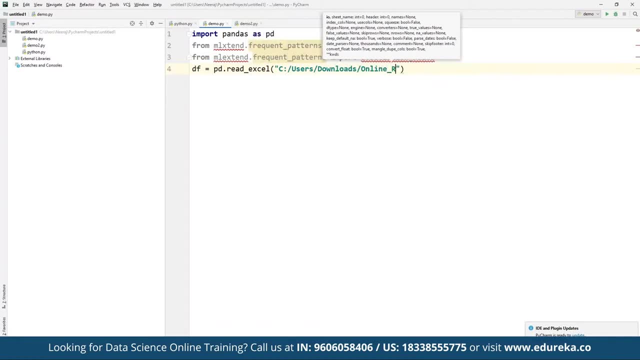 and by the name of online underscore retail dot excel s6. so this is the reader we have currently imported here and, in case, suppose, some libraries are currently missing here, so we can import these libraries as and when required here. suppose if we, if something is missing here, we can simply import these libraries in case they are not properly installed. 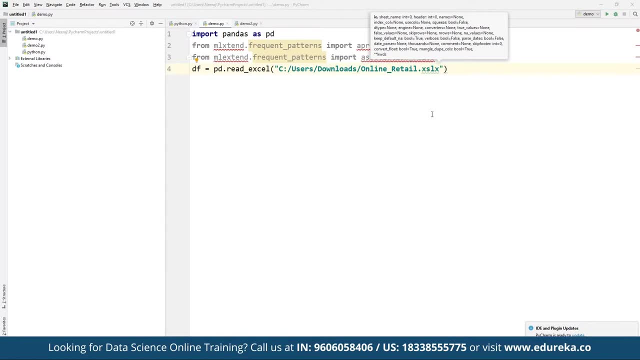 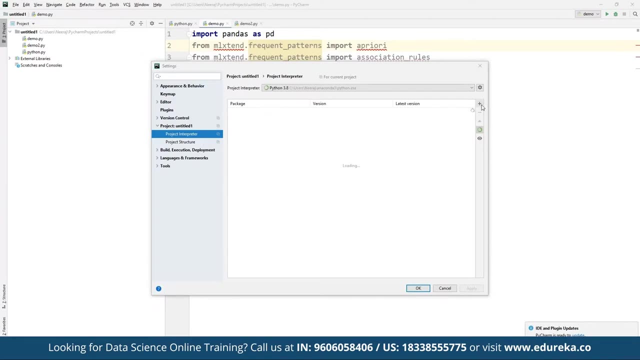 so for installation of any new library here we can go to file under settings. here we have to go to project interpreter in case you want to add any specific library here, then we can simply import the library here, and then we can import the library here, and then we can. 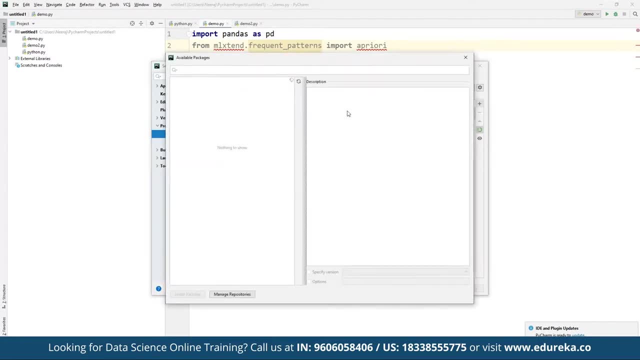 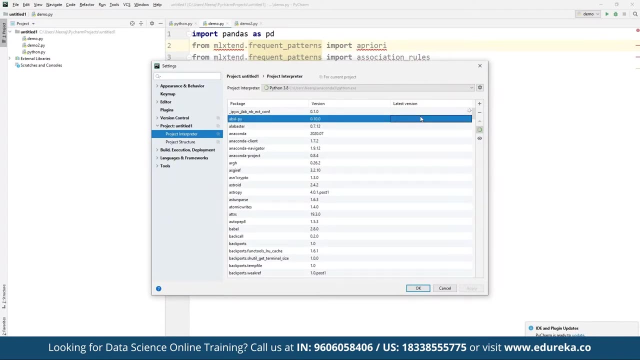 simply click on plus and then we can choose which all library we want to add. here we can simply see the entire list of all the libraries currently installed here and now. if we want to start with more, then we can simply add more libraries and then we can start deploying it one. 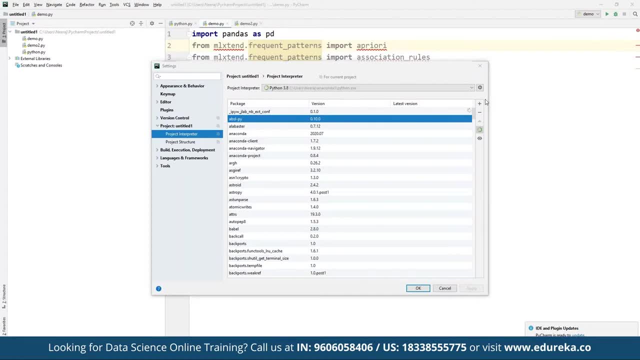 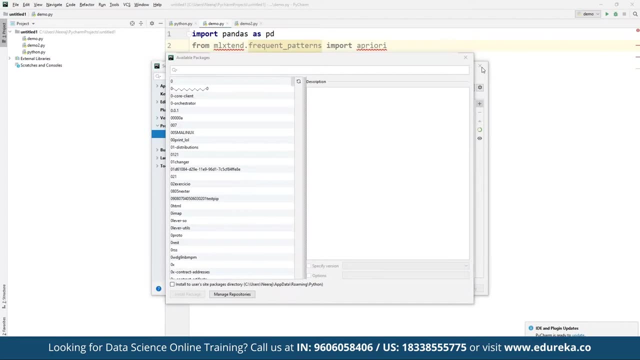 by one. so for example suppose, if we want to install any specific library here, so here we can. so let's say, here we want to install the apriori here, so we can see, here we can also import the ms train. so if this library is installed here we can also import the ms train. so if this library is. 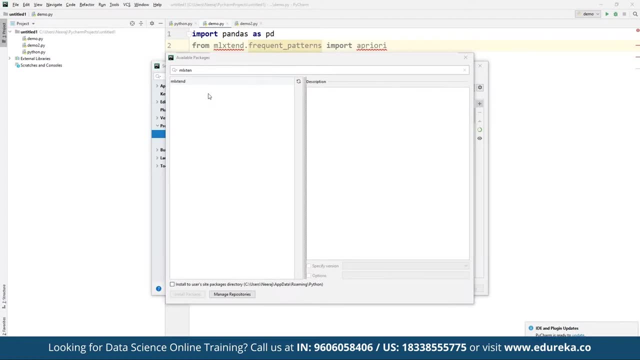 currently available. we can simply click on install package and this is going to be installed and stored in a system as a library. same way, if you are looking for apriori here, so here we can also use, because again, at the end we are going to use apriori from the ms train that we have imported. so 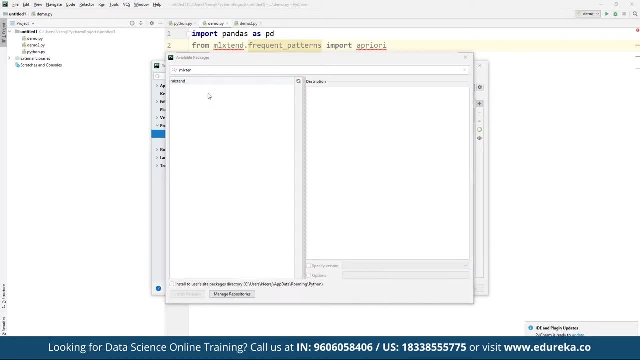 here. we are going to install the other package as well. so the first package for ms train has been installed, and now we are. and now if you want to install the other packages, then we can also install it. so if you want to install the other packages, then we can also install it. so if you 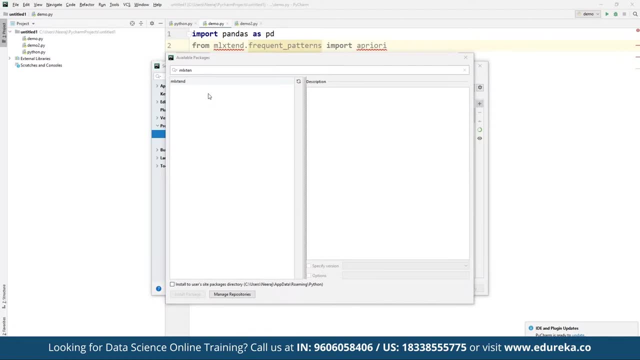 in case we have missing some kind of library, then we can simply install it. or in case we are, we have not used those libraries here, then we can simply use them one by one. so once we are done, we can simply come out. so, as you can see, now, once the libraries have been properly installed and we 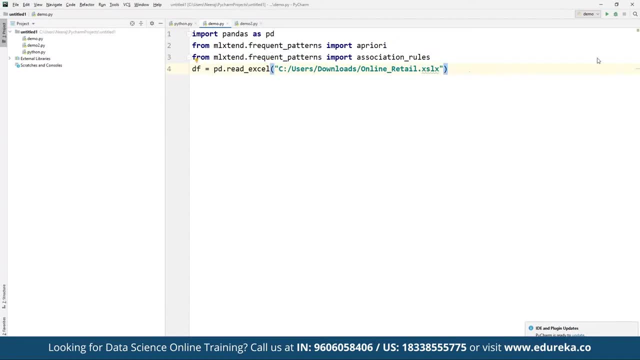 will see. there is no error being shown here. and this is the path of the file where we have stored online's retails dot xls file here. so just to confirm, we can confirm that we do have the file by the name of online retail dot xls x available here in a download directory. so once we have specified the file here, 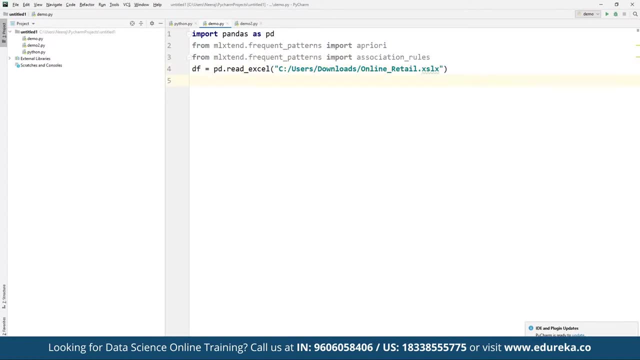 and then we are going to simply use data frame, dot head. so in case we want to see the first few entries of the current data set that we have imported, so here we can simply define dfhead and then, from the given path, the first two head are is going to be returned back as a response. 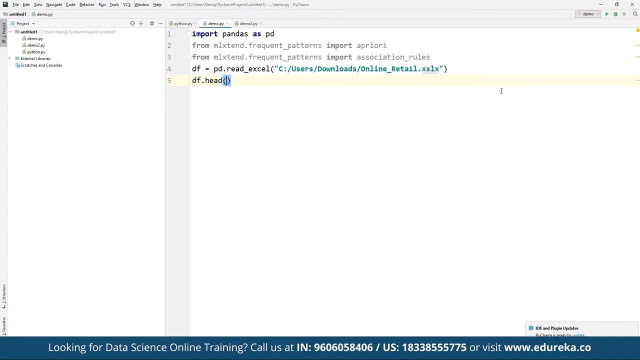 now. once we are done, we can simply start applying it now, once we have the access to the data set here. next step is going to be focus on data cleaning, which will include removing spaces from some of the descriptions that we have, and for that we are simply going to specify here we can, instead of 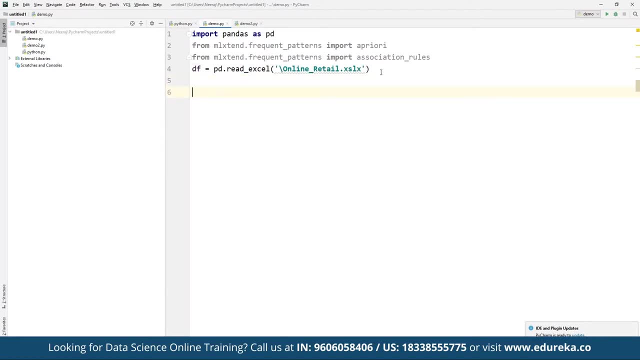 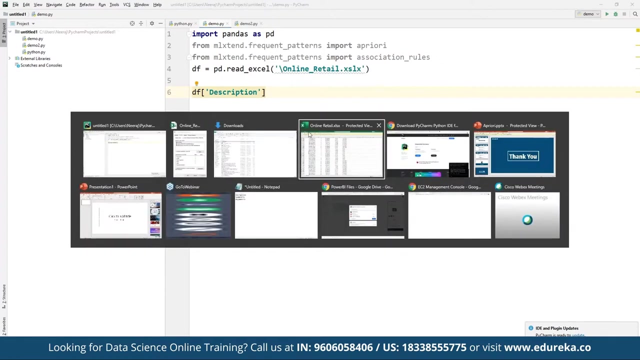 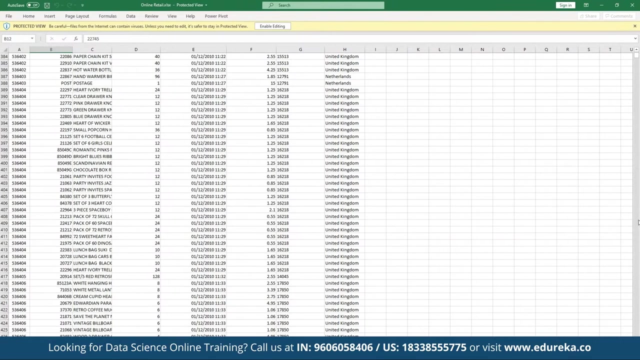 using the data, the data frame head here. so now we are going to use the data frame and then from here we are going to add a short description. so here we can add a short description here. so basically we are just using as data frame hot to go through and from here we are His listed an. 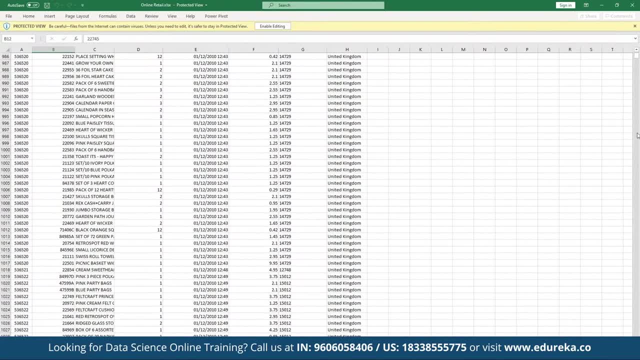 example. so here we have the data adopt ing or fit present His list of spaces. those are different descriptions of when I need to remove Renee somewhere in the exam panel or when don't need it for skipping to theprobout tables, as well as replaying the file address and the state. likeвод aparig. 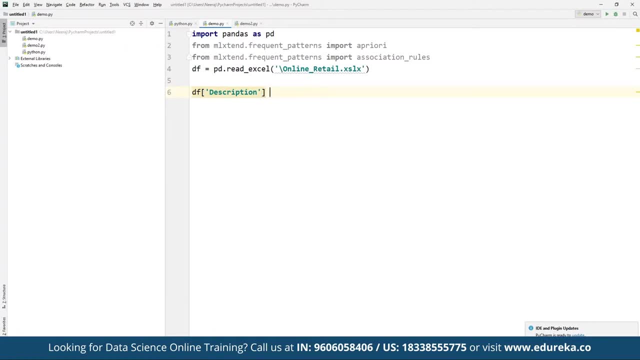 we have to work on removing those kind of anomalies. so here from the data frame. so here we can add parameter as description. now, under description, we are going to use the string function as string dot strip. so string function is available under string. we're going to make use of it. 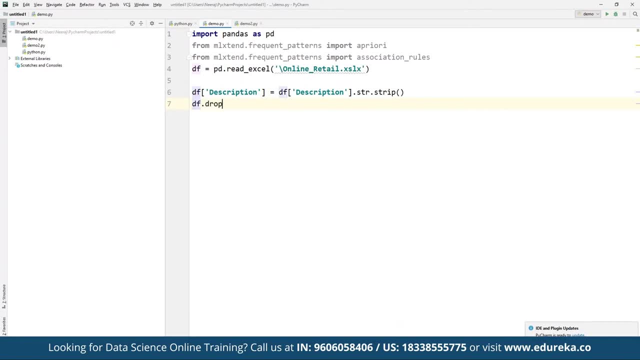 and then same way from data frame we are going to work on dropping. there we can find the values for x is equal to 0, and then the subset where the. what kind of values we have to drop? do you have to define that parameter? where the invoice number is going to be in place is going to be true. 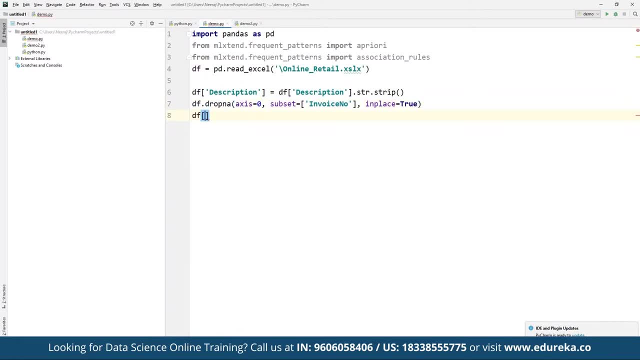 and then from data frame we can define the invoice frame, the invoice number, and then we can define it to be our data frame. where invoice number: again we are going to convert that to a string itself. so here we can define data frame and then the invoice number type. so here we have invoice number. 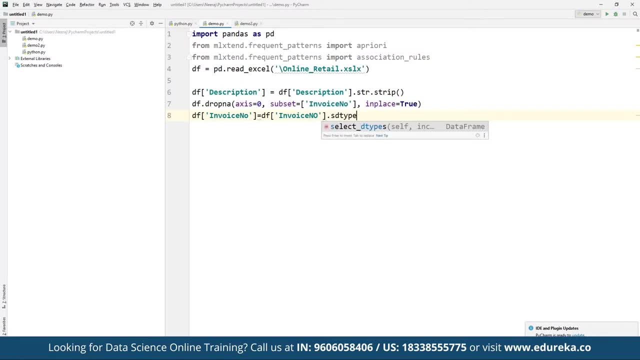 dot the as type, and then we are going to the sd type here. but again, here we can keep it to as type. so here we can define to be a string value, so here we can find to be a string, and then we can create a data frame where we can find data frame. 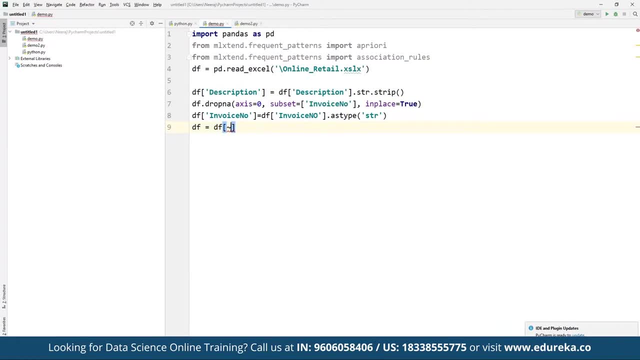 should be a value closer or get a value closer to data frame where we are going to define the invoice number. so here we have invoice number and then we can define this as a string point. we missed on the, so here we have string dot contains and then we can define wherever. 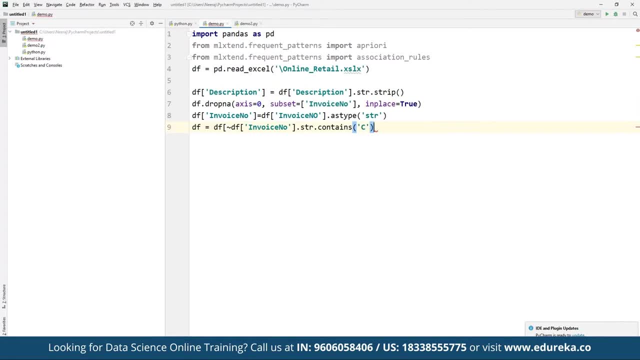 the value is c, wherever the value is c as a power definition defined here, and then we are going to simply save it as a part of given data frame. so after we are done cleaning up, we need to consolidate the items into one transaction per row with each product. so for the sake of keeping the 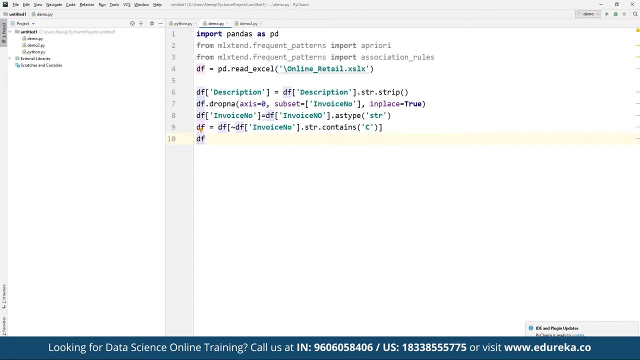 data small. we are only going to look, we are only going to be looking at the sales for the for any specific country. so now, once we are done, we are going to create and consolidate the items into one transactions per row with each product and, for the sake of keeping the data set small, we 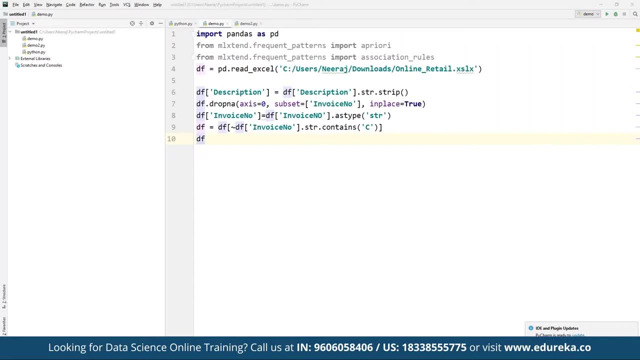 are going to look at the sales for a specific country. so for that, let's say, here we want to focus on one country, data set here. so here we can use basket and then in the basket part, here we can define multiple data frames. for example, first of all we can define data frame and here 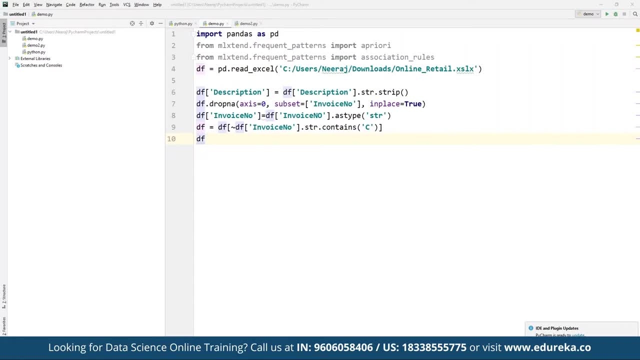 we are going to use the same data frame and then we are going to segregate it further based on the country itself. so here we can find country and then under country we can define which country we want to focus on. the country should be, suppose, let's say, we want to focus on the country itself. 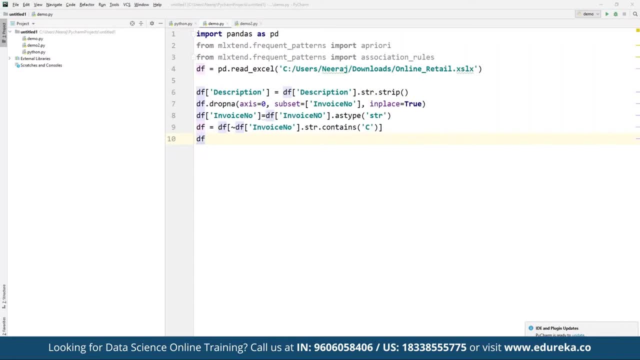 say france as a single country. so here we can define france as a country that we want to use for consolidation. and then we are going to group. so here we can use group by the invoice number. so here we are going to find the invoice number for it. so here we have invoice number and then we can. 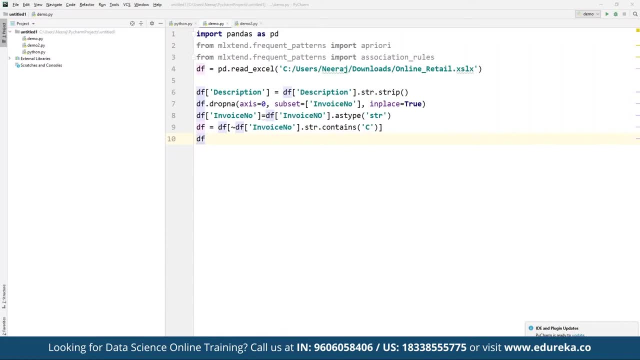 add a short description here. so here we can add description, and then, after we are done defining the description here, we can then define the quantity here. so here we can define quantity, and then after quantity we can define sum. let's put this underline, just to what the confusion? so here we can define: 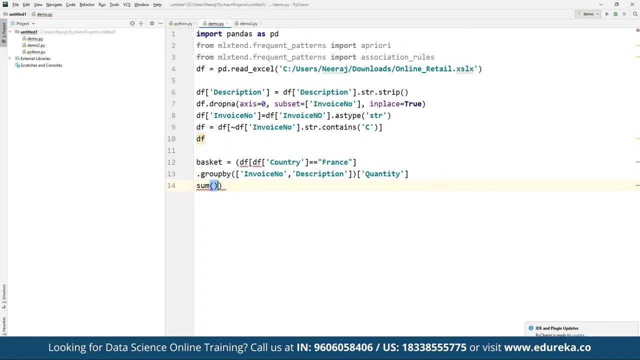 sum, and then we can define unstack, dot reset. we missed one of the advantages here, so here we get to. here we have to define sum and then we have defined unstack, and then we have to find dot reset, dot reset and then the index value here. 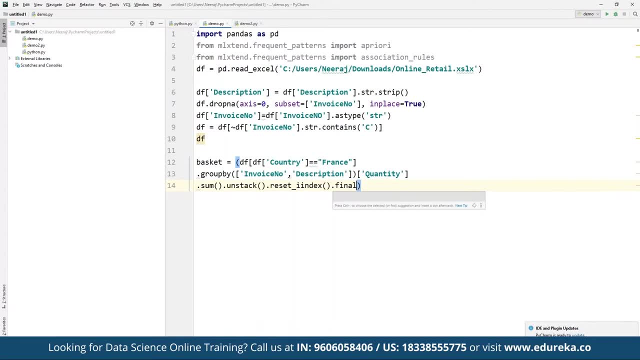 with the final, any with the final, or consider the simple fill, color with the simple fill, and then we can define it, the value, to be a simple zero, and then we can use set underscore index where we can define for the invoice number. so here we have invoice number defined and then we can define this for a basket. 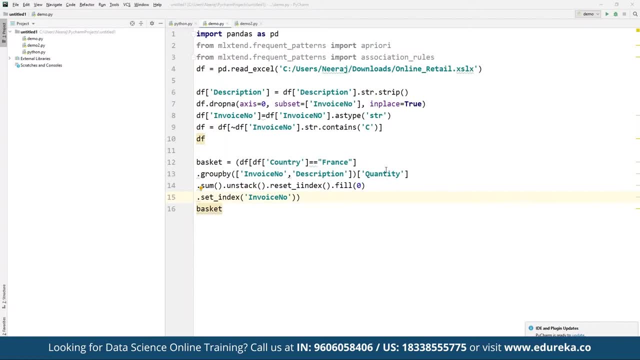 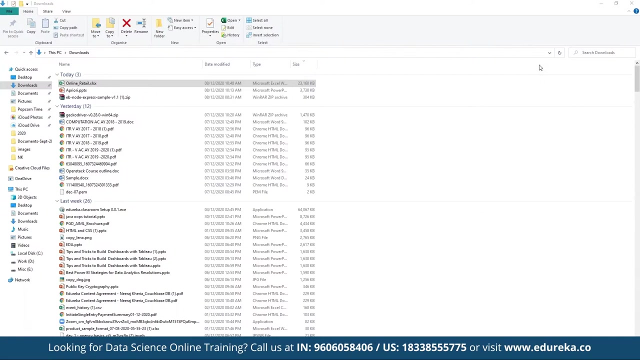 so basically, here we are going to define the consolidation for the items into one transaction per row with each particular product and to keep the number of transition low. we have we have focused our attention only for a for single country, so as in france. so afterwards, so after we are done with that part, next we have to work on removing all the zeros. so 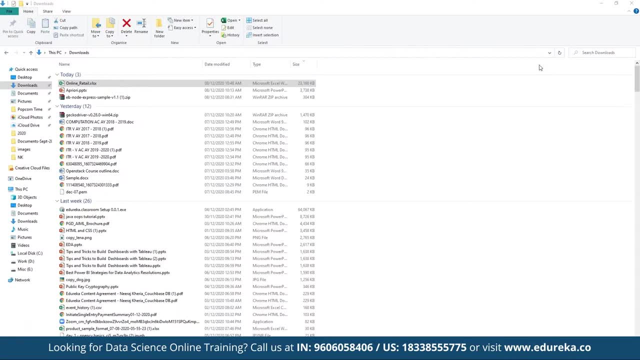 basically, there are a lot of zeros in the data, but we also need to make sure that any positive values are converted to a one and anything less than zero is also set to zero. so for that we are going to make use of this. so, basically, here we are now for converting that. here we are going to make. 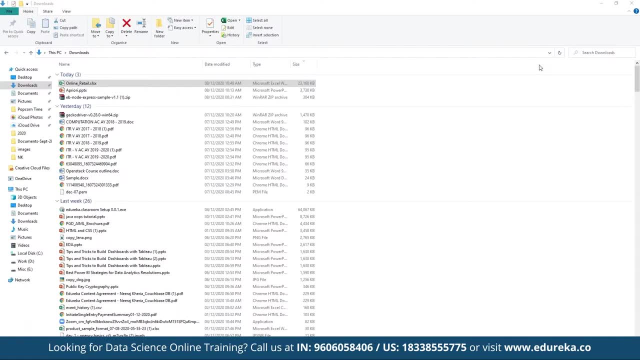 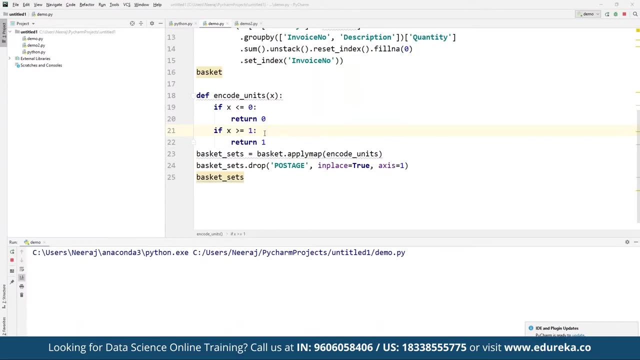 go ahead and perform the encoding. so here we have a teacher. ahead and perform the encoding. so here we can define encoding units. so if x is less than or equals to zero, then we are going to turn zero, and if x is greater than or equals to one, then it is. 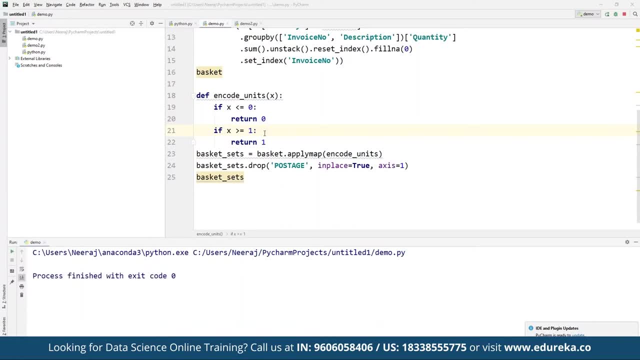 going to turn one where we are going to define the basket sets and the basket apply map encode units, and then we are going to simply use the drop postage and place setter to be true here. so basically, here we are going to simply work on, first of all, removing all the anomalies here. 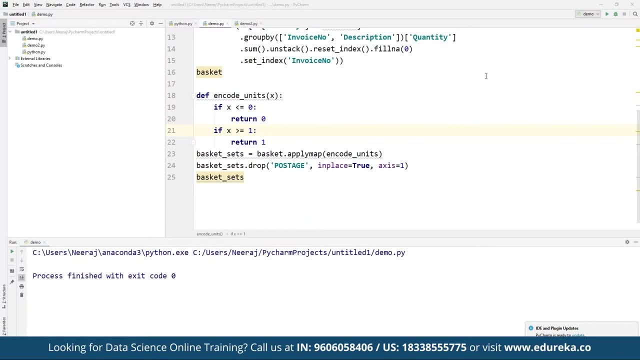 and then, if there are a lot of zeros in the data, we also have to make sure that any positive values is converted to one, and anything less than zero is all this up to zero. that's what we have done here, and then we are going to generate a frequent item set that have support value of at least. 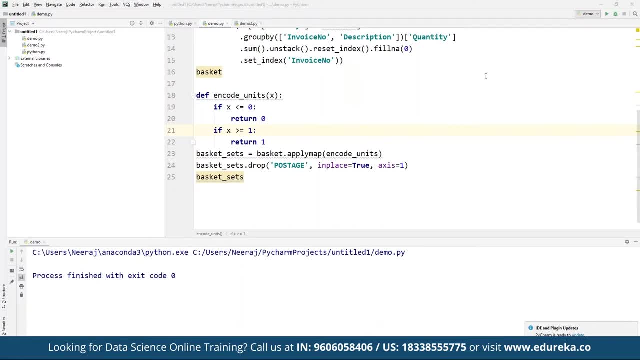 seven percent, and this number is chosen so that we don't, so that we can get close enough and we don't observe any kind of errors. we or we don't. you get any, it any errors thrown, and here we can generate the frequent, generate the rules with the corresponding support, confidence and lift. so for doing that we can make. 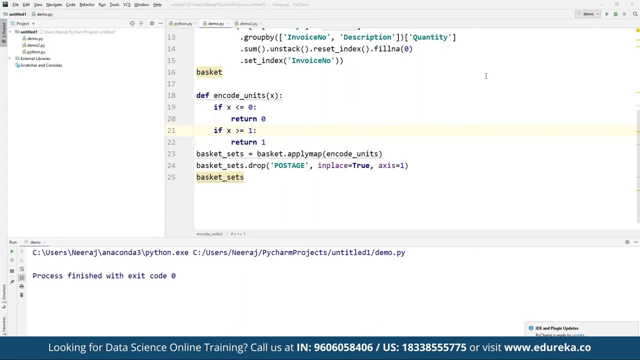 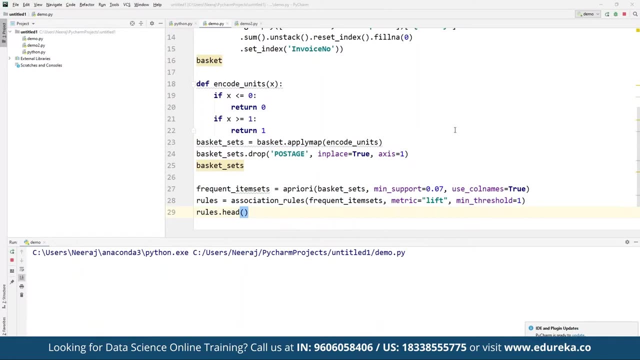 use of frequent item sets. so here we are going to find frequent, frequent item sets where we are going to find the a priori from basket set. minimum support should be 0.7 and the call lengths that are going to be used is should be true and the rules here defined should be for also. 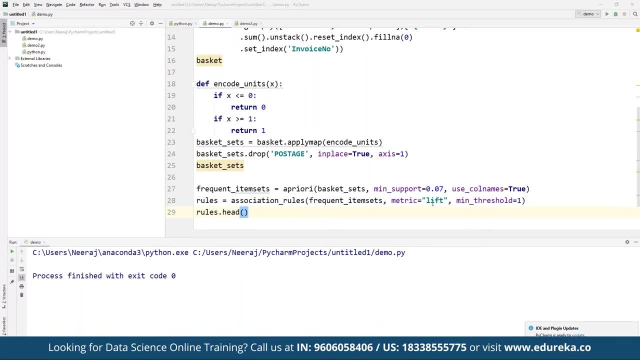 be a kindergarten set set. click on first, on the next and finally the fifth fit by method. okay asks for what does the test run on with this machine? and here we are going toям notice that the best put is answer: using machines that are working on this machine. looking at specific services, customers, we are 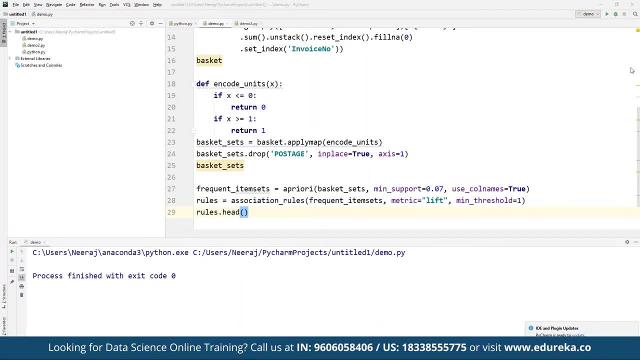 measuring herself by making use of the integration statement to show us that we can print activity. so the Cantor of things been fácil para completar y leamy el producto chics Debra. I need to say if we are looking for things, for something, it depends on the type or availability of another thing. this: cannot be us. this hand signs to the user, so the setting status is variable. so we can create, or Giama that I will show how. if we're working on this, we're going to look at that. now there's no particular button, but we're going to see. does it look something like a single event, like, and you find that the view can see? 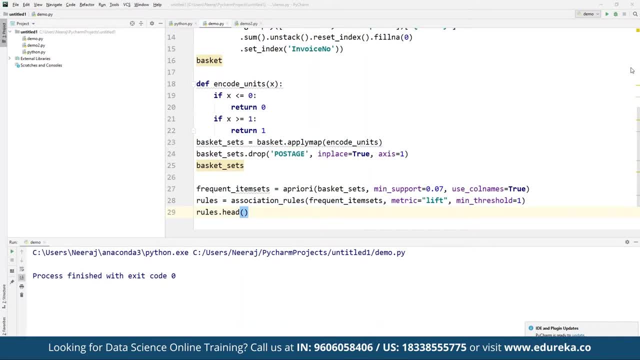 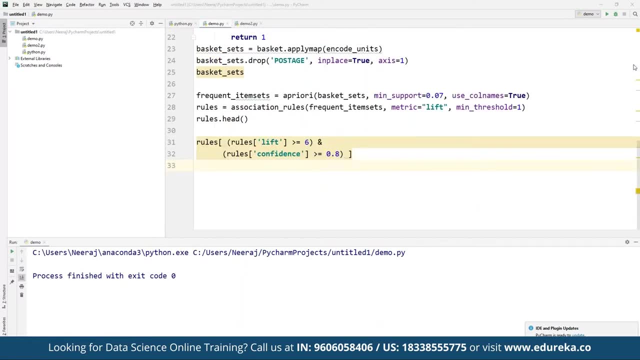 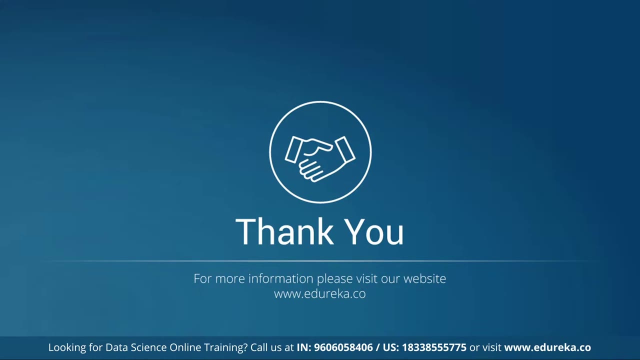 is going to be defined as a value greater than 6 and the rules fair confidence value is going to be 0.8 altogether. so that's how we can make use of the a priori algorithm here. so, as it's almost time now, so let's do one thing, let's say we wrap it up for today, guys. thank you.